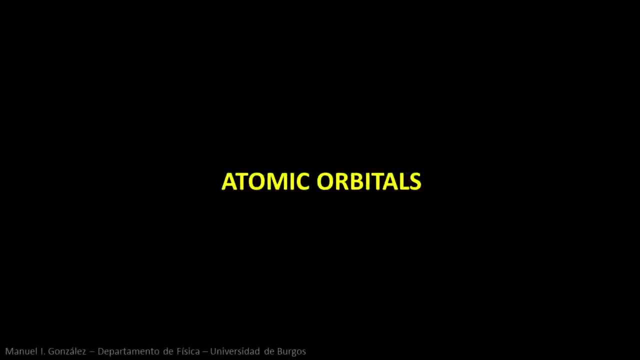 This is a semi-classical picture of the lifeless atom hydrogen. An electron describes a circular orbit around the proton In the lowest energy state. the radius of the orbit is the so-called Bohr radius. This image is inaccurate for several reasons. 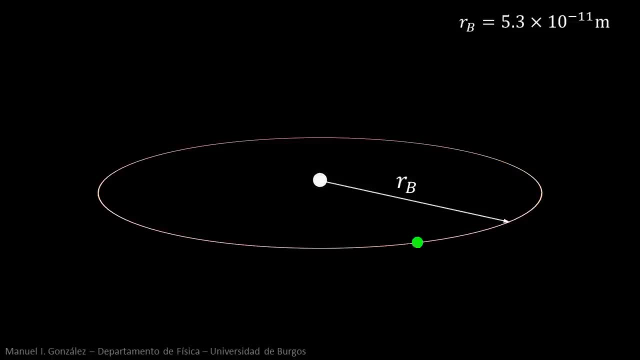 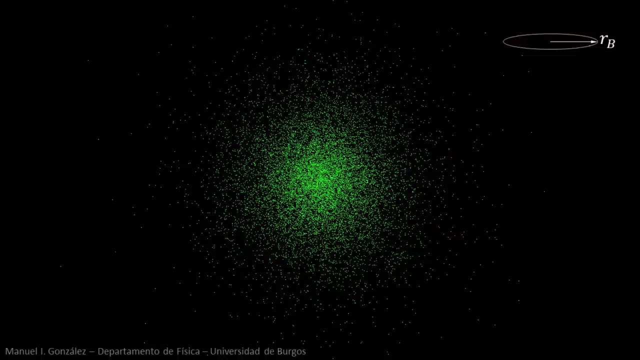 First, the size of the proton is about 50,000 times smaller than Bohr radius. Second, quantum mechanics teaches us that the electron is not confined to a well-defined orbit, nor can it be located accurately. Instead, it occupies a region of space around the proton, called orbital. 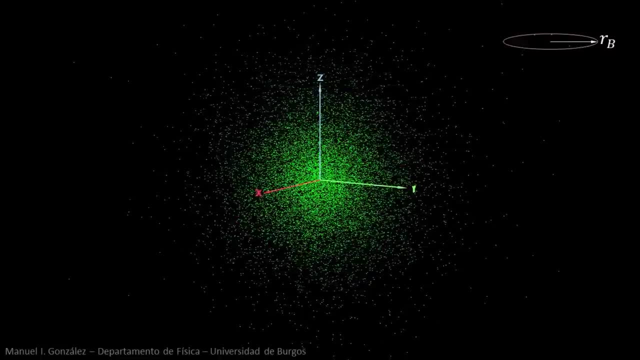 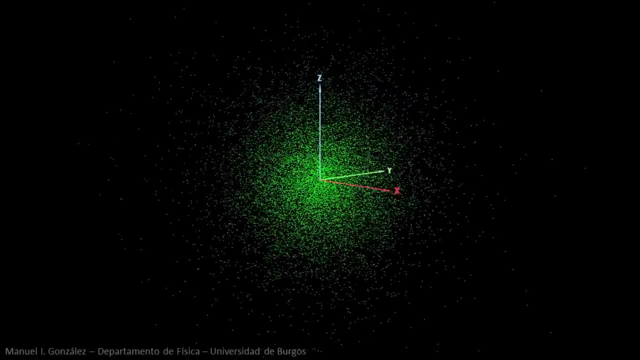 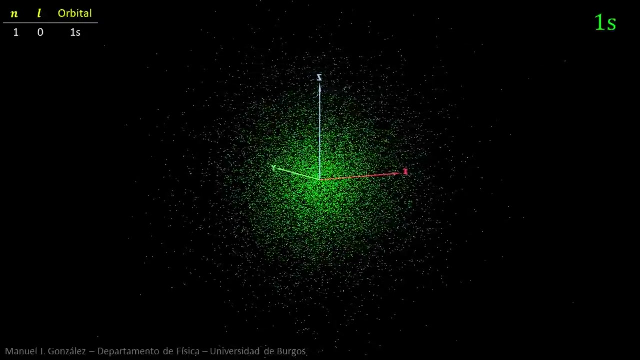 This simulation depicts the orbitals as clouds of points. The regions with the highest density of points are those where the electron is most probably found. The ground state orbital is called 1s. The 1 is the principal quantum number which is related to electron energy. 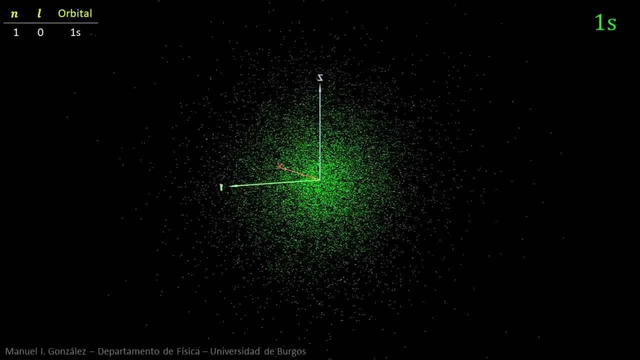 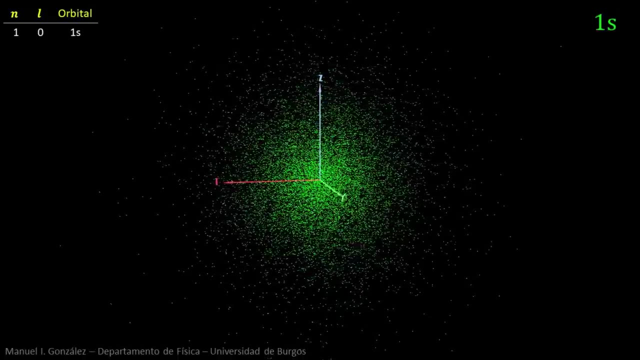 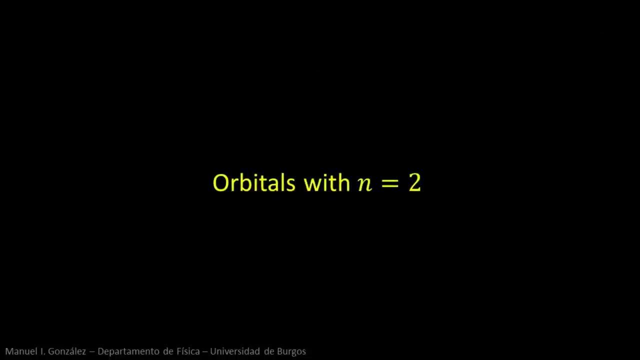 The s means that the orbital quantum number L is equal to zero. S orbitals have spherical symmetry, so the probability of finding the electron does not depend on the direction. S orbitals have spherical symmetry, so the probability of finding the electron does not depend on the direction. 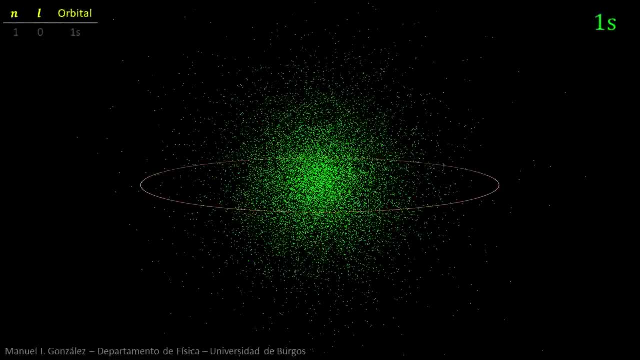 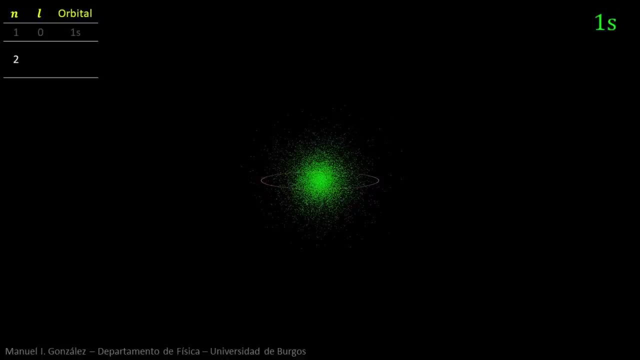 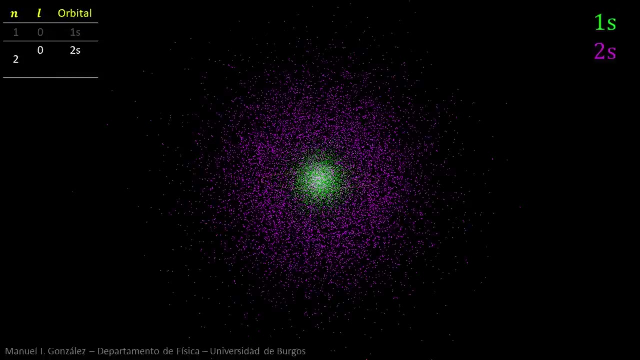 The radius of the second Bohr orbit is 4 times the Bohr radius. Therefore we must zoom out. Quantum level 2 comprises two values of the orbital quantum number. Orbital 2s corresponds to L, equals zero. As we see, this orbital occupies a much wider region. 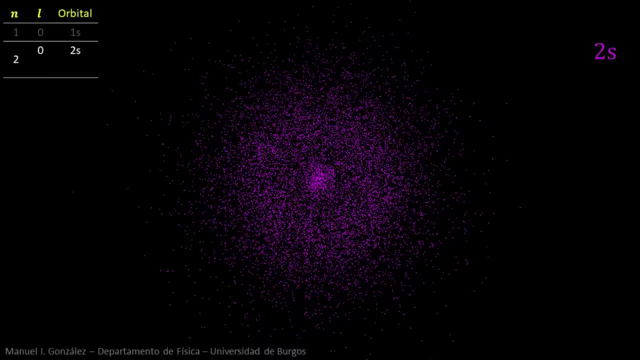 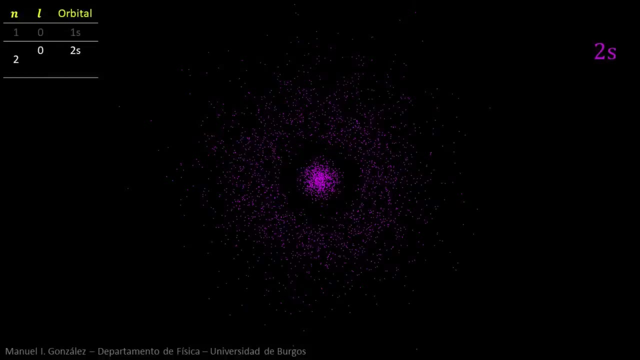 Let's make orbital 1s disappear and display only a thin slice of orbital 2s. In this way, we notice a radial node, a distance at which the probability of finding the electron is zero. Again, this is the full 2s orbital. 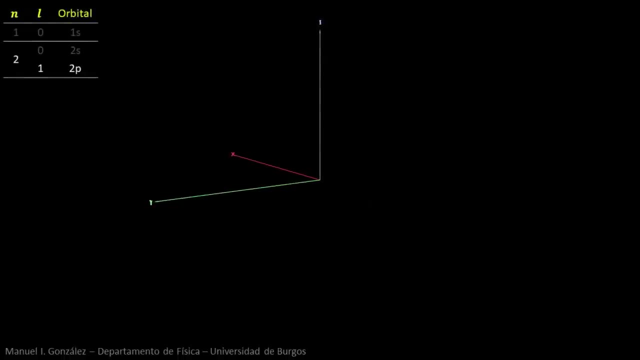 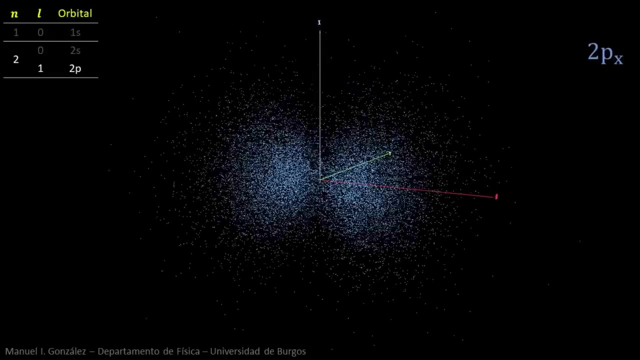 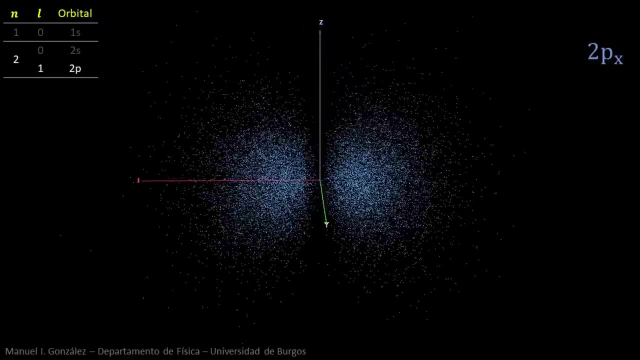 Quantum number L equals 1, gives rise to three orbitals called 2p. This is one of them. It consists of two lobes which we can consider aligned along the x-axis. The second one, 2py, lies along the y-axis. 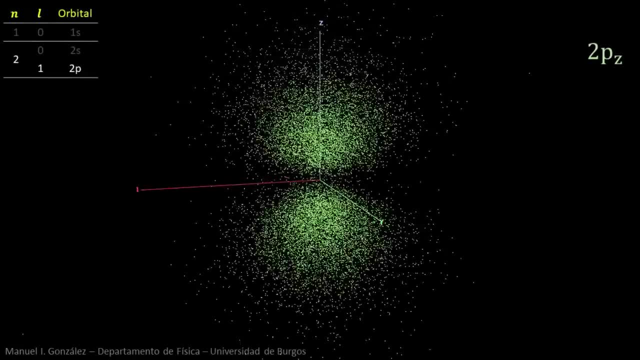 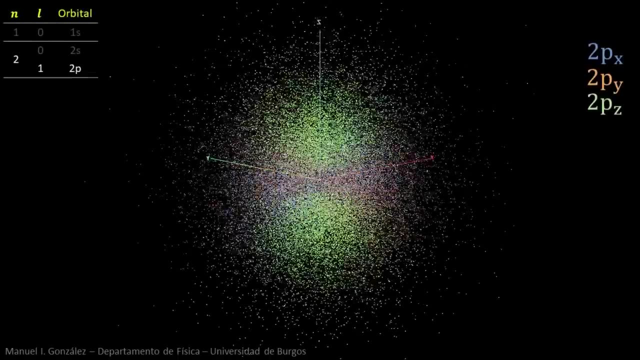 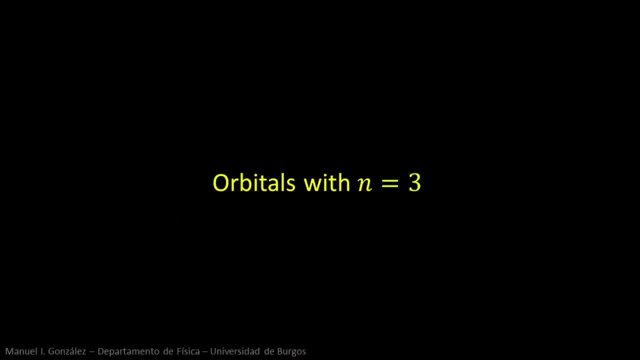 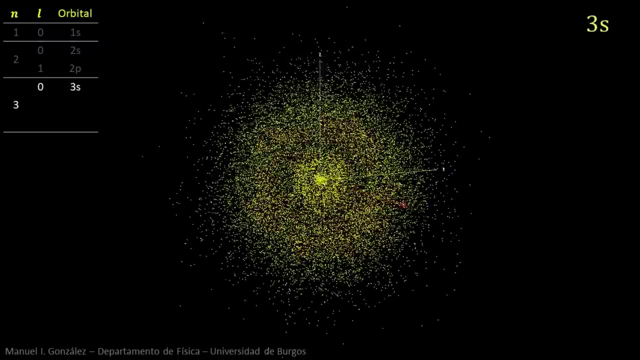 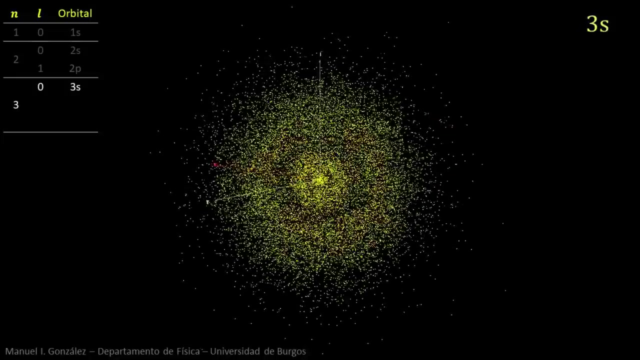 Finally, this is the 2pz orbital. If we display all three orbitals at the same time, the complete electronic cloud becomes somewhat confusing but shows a high degree of symmetry. The third energy level allows three different Ls. Again, 3s orbital corresponds to orbital quantum number zero. 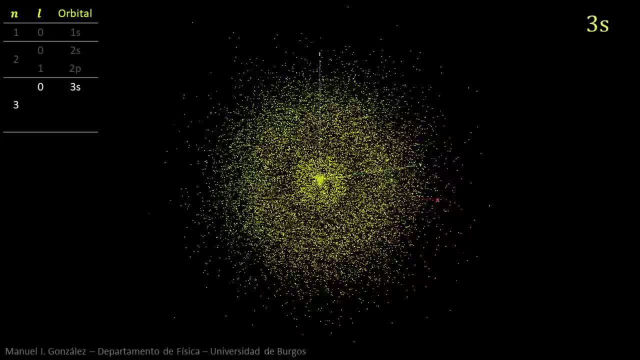 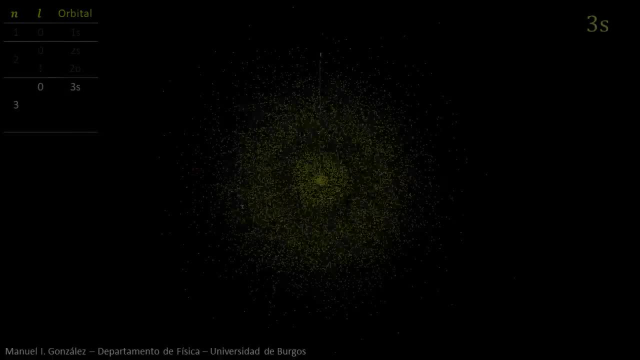 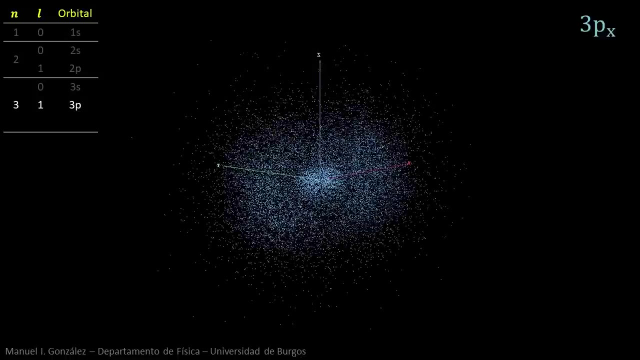 It has two radial nodes. The outer one is clearly visible in this scene. The inner one is hidden by the surrounding cloud. Just as 2p orbitals, 3p ones have dumbbell shape, but with a radial node splitting each lobe. 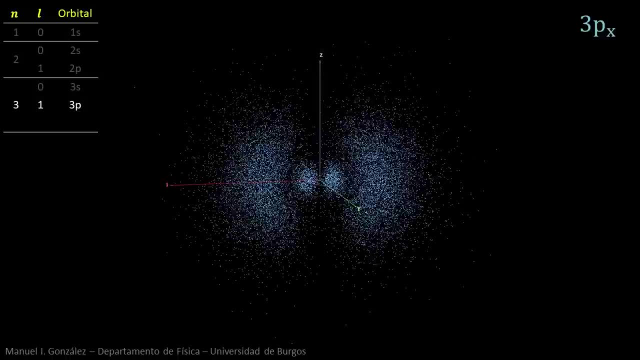 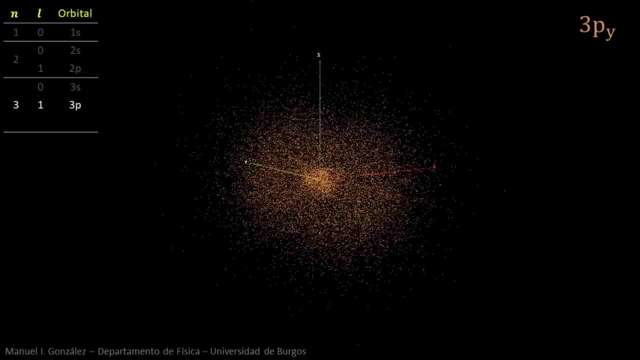 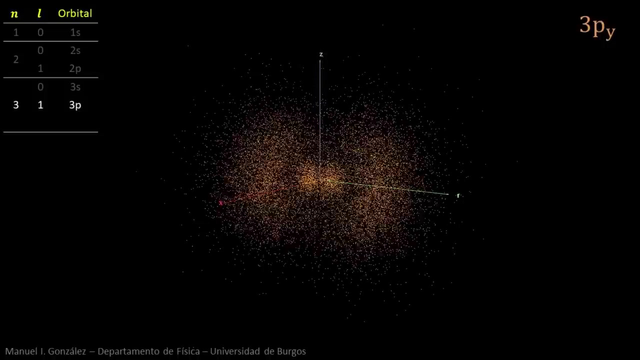 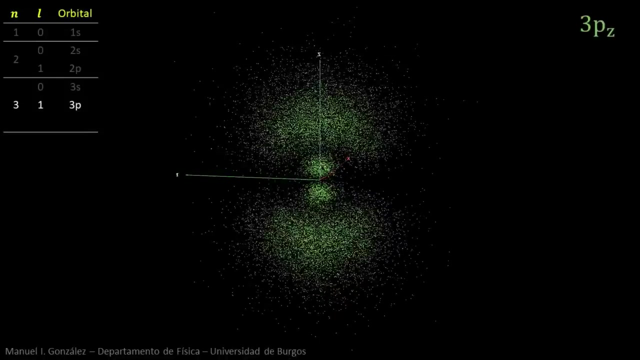 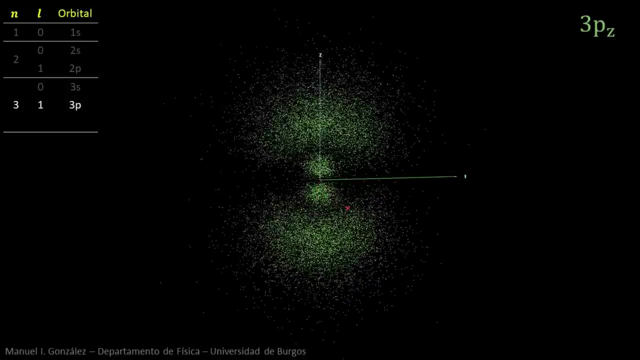 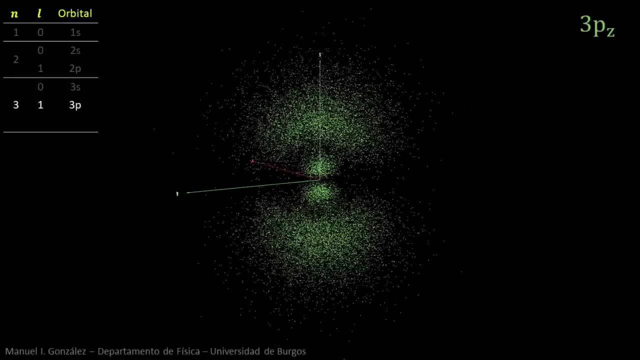 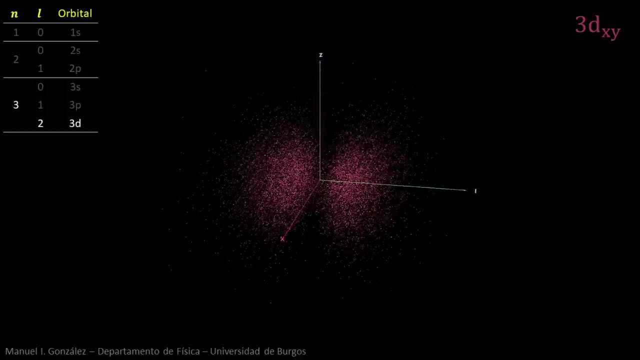 This is 3px, This is 3py And 3pz. There are several ways to choose the five 3D orbitals. This is the most popular one. Three of them have four lobes bisecting the coordinate axes. 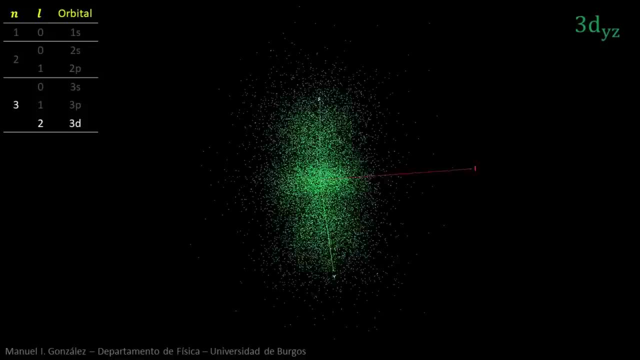 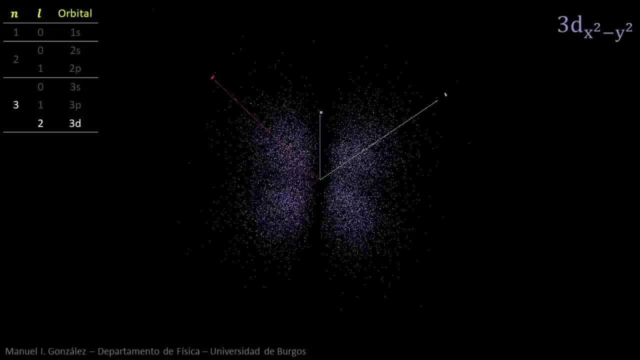 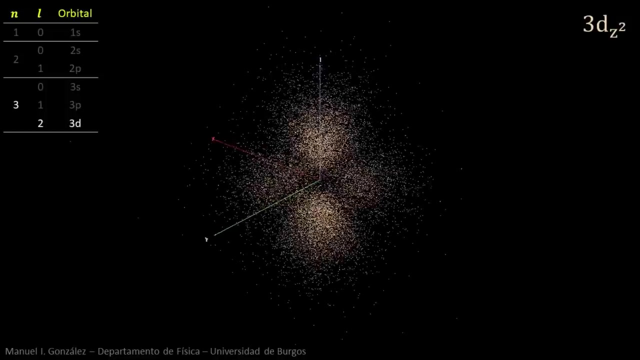 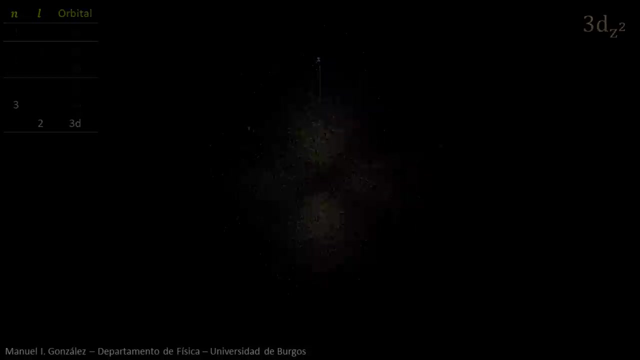 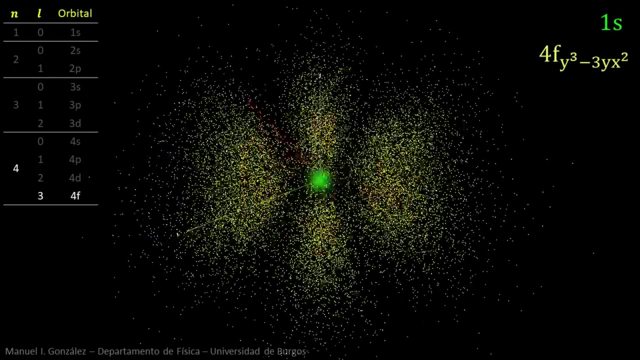 The fourth one has four lobes along x and y axes. Finally, the fifth one has two lobes along z axes and a ring-shaped region on the xy plane. As quantum numbers grow, the orbitals become increasingly complex, in shape with new lobes. 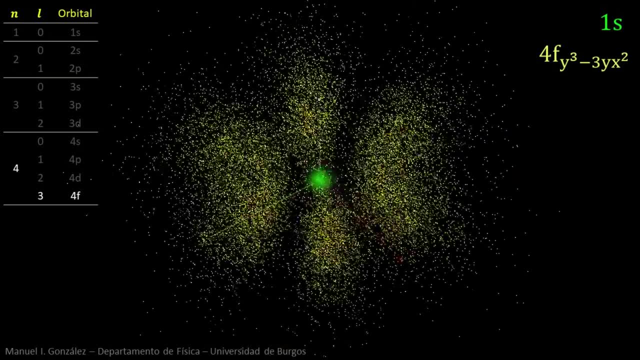 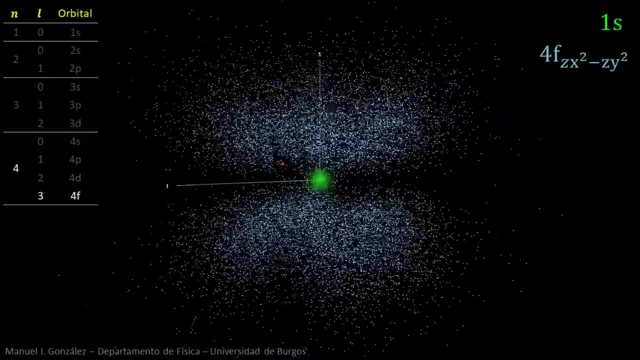 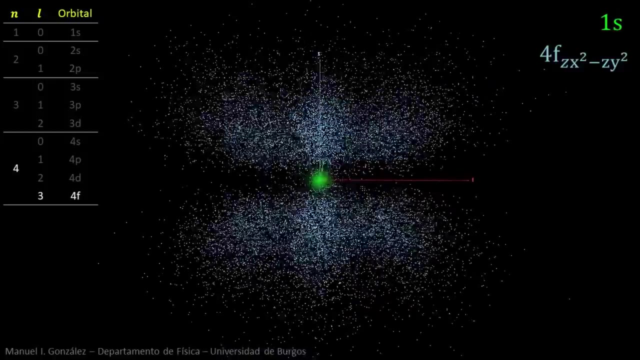 and nodes. For example, this is one of the seven 4F orbitals. This is one another. The average electron-nucleus distance also becomes higher and higher. Notice the difference in size with the ground state. 1S orbital. 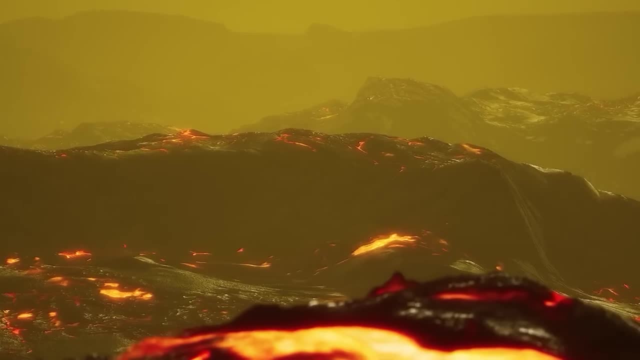 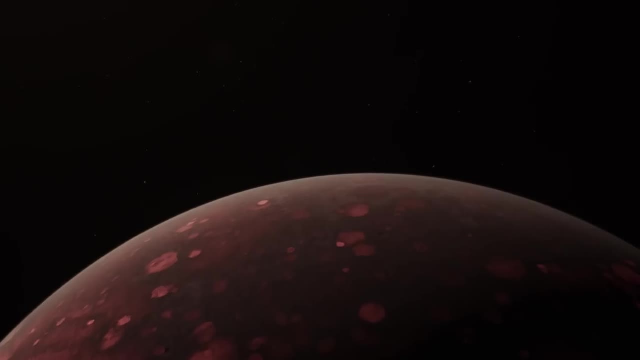 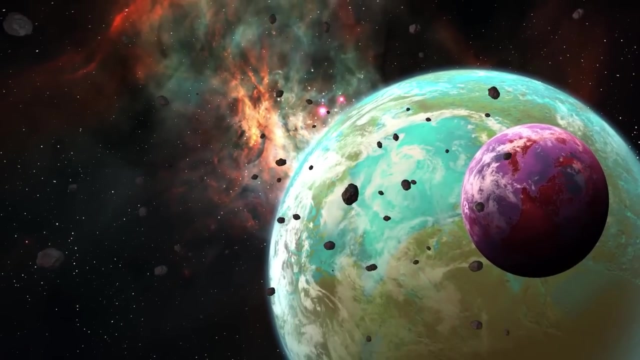 See. this structure Looks scary and devoid of any possibility of life, But this is our home: the Earth at the beginning of its existence 4.6 billion years ago, And its formation and the formation of the Moon remains a mystery. But today we'll tell you about the theories. 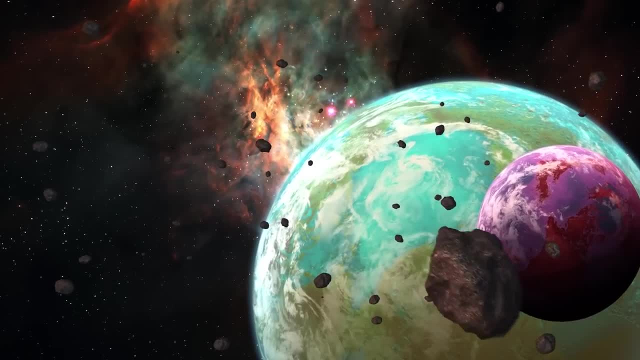 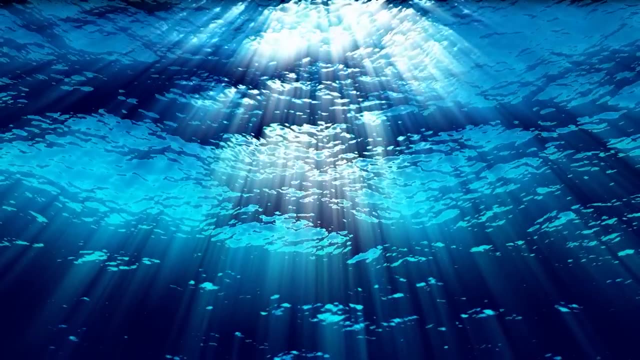 that scientists suggested. You'll learn how planets so different from each other form from the same material, what planet crashed into the Earth in the past, how much water there is on our planet and where it came from. And, finally, we'll tell you how old the oldest organism on. 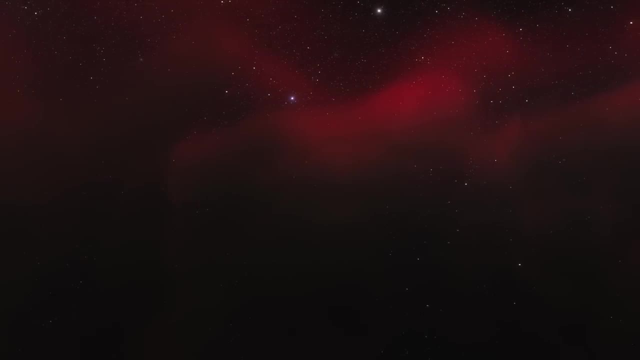 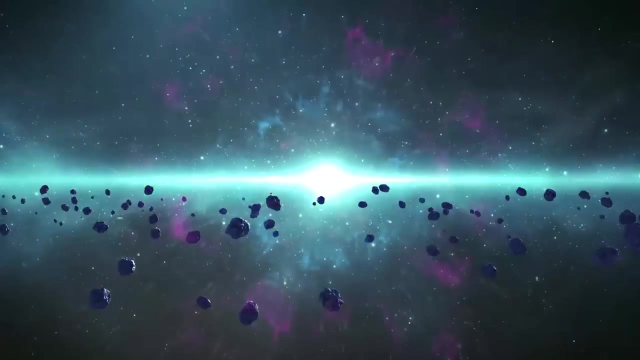 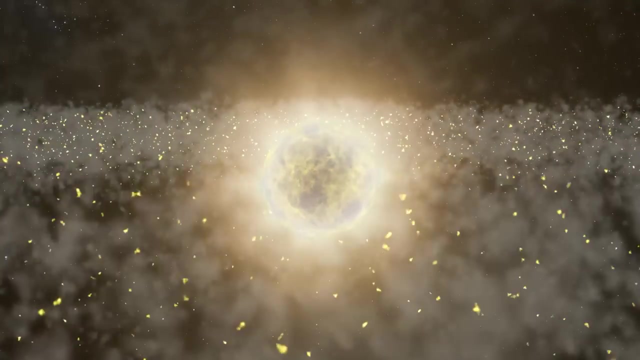 Earth is. We prepared the story of our planet from a clump of dust and gas a few miles in diameter to the appearance of life. When the Sun was created, gases and other materials around it started colliding with each other and forming small bodies called. 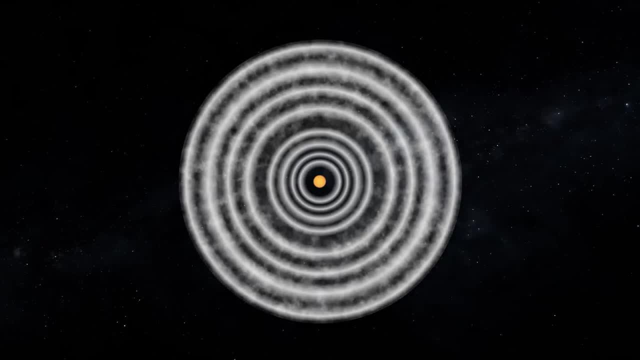 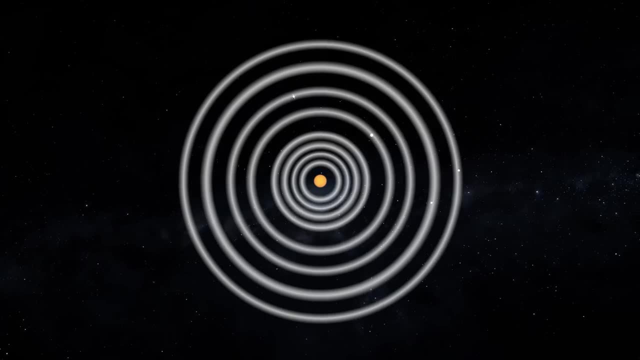 atoms. When the Sun was created, gases and other materials around it started colliding with each other and forming small bodies called atoms- planetesimals- And as the gravitational forces were growing, more material was pulled together and these seeds of planets grew larger until they became true planets, The solar systems. 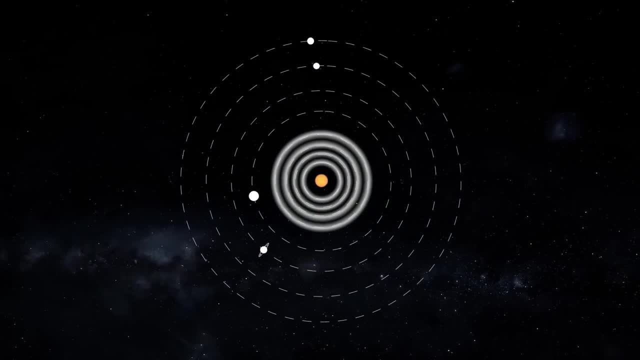 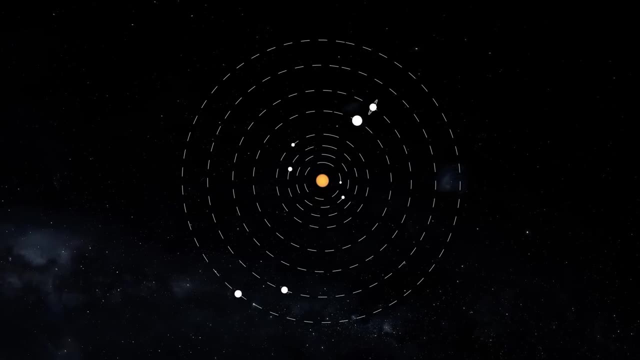 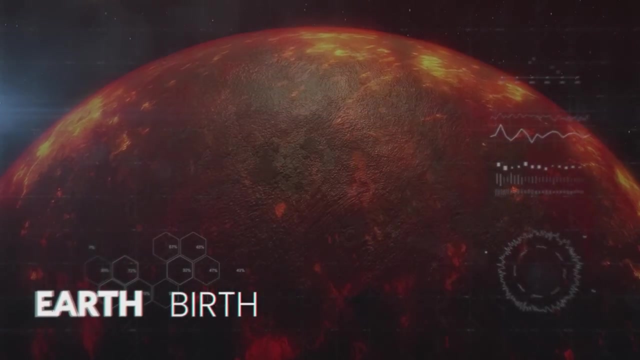 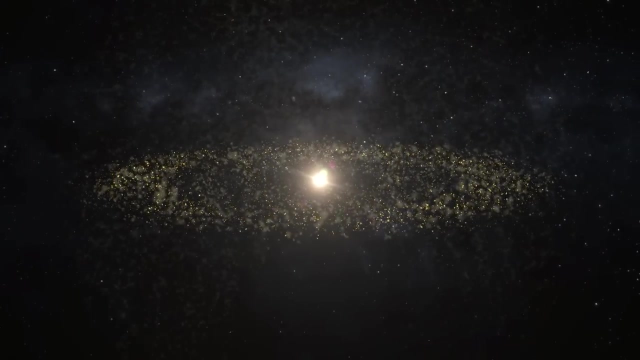 gas giants Jupiter and Saturn, Uranus and Neptune were born much earlier than the four known terrestrial planets Mercury, Venus, Earth and Mars. But how exactly was our home planet born? The Earth's story started about 4.6 billion years ago in a disc-shaped cloud of dust and gas rotating around the early Sun.